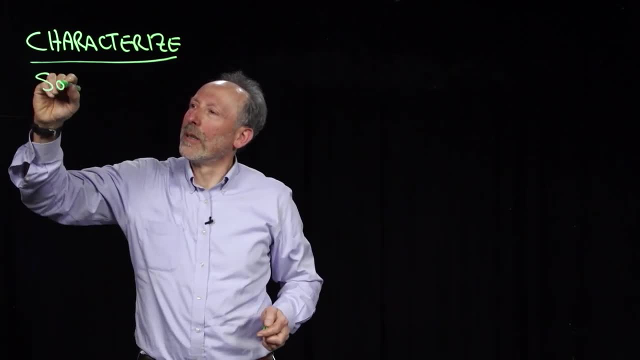 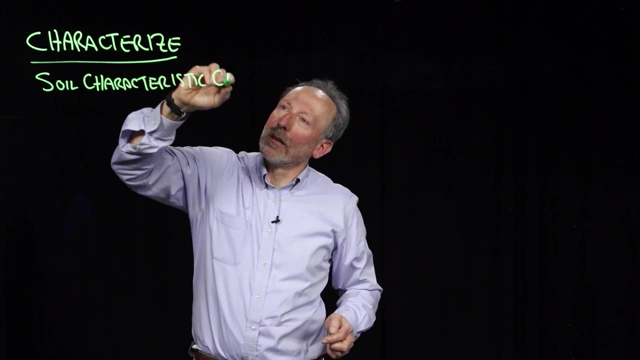 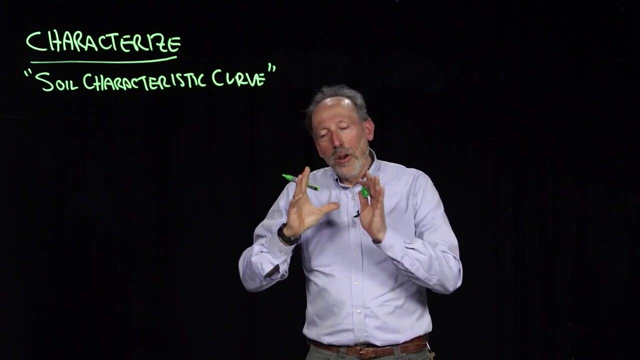 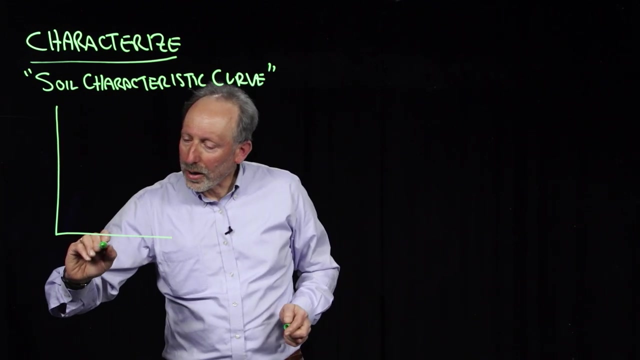 the soil is. we're going to use the soil characteristic curve, The characteristic curve And what that is really trying to do is identify how water is retained by soil. So what we're going to do is on one axis, we're going to put the water content. 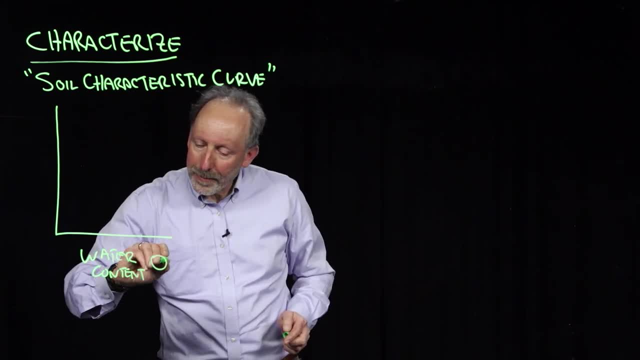 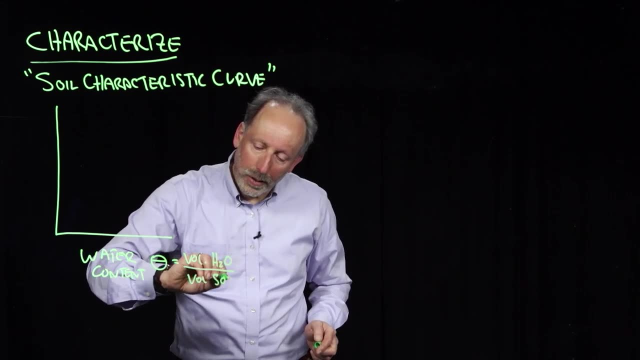 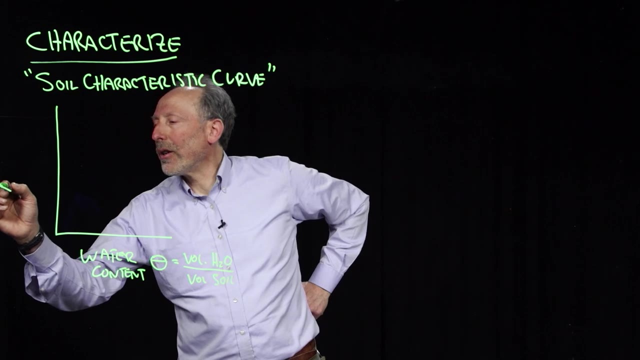 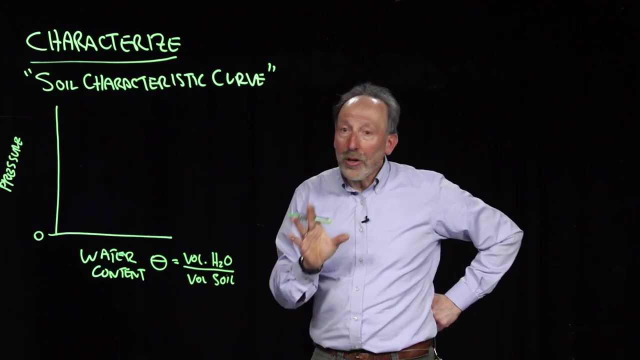 And we'll use the symbol theta, which is the volume of water per volume of soil. You could also do this in terms of the mass of water per mass of soil. On this axis we're going to put the pressure And we're going to start it at a pressure of zero And at a pressure. 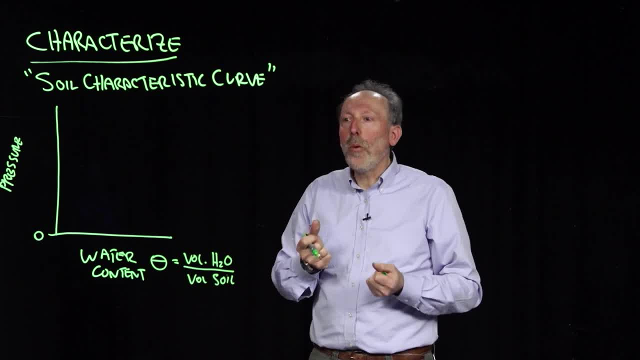 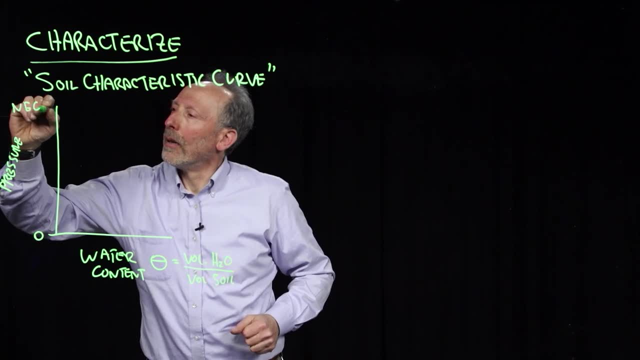 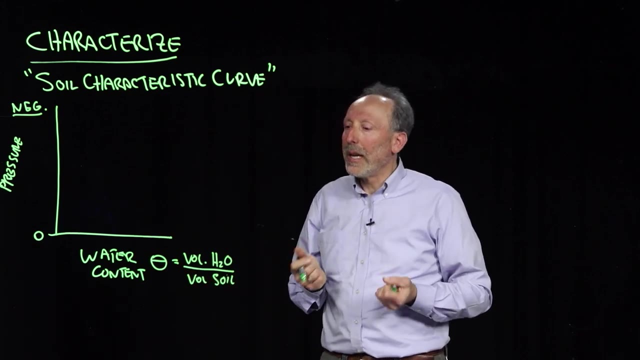 of zero. the soil is saturated, That means that there's no tension pulling water out of the soil- And notice that we go negative pressure at the top. So we're going to go from zero to more and more suction or negative pressure. So what we have on this curve we start with. 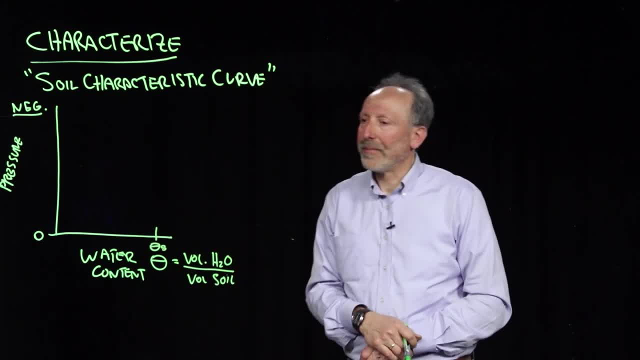 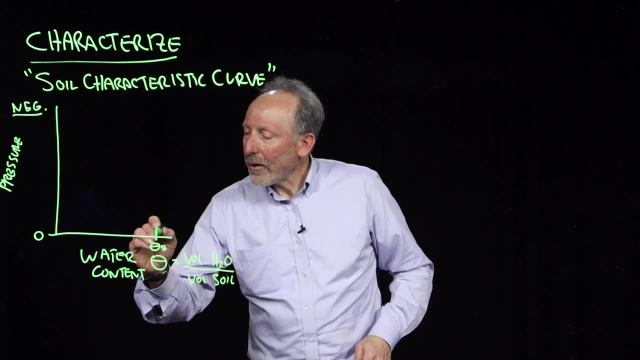 when it's saturated, we call that theta sat. So that's going to be the theta sat, And that's going to happen at zero pressure. And then, as we drain our soil, we're pulling the water out. it dries, And so it dries. 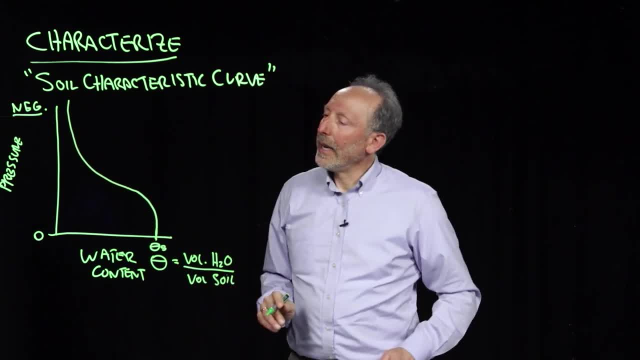 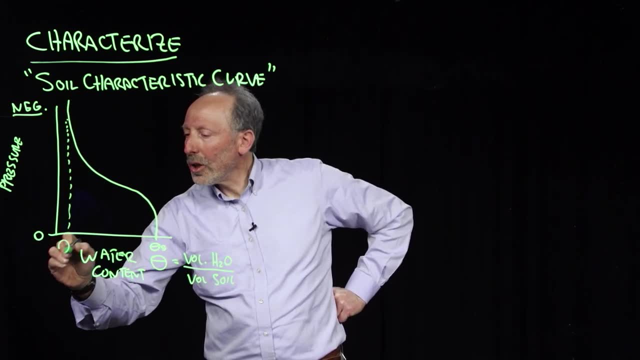 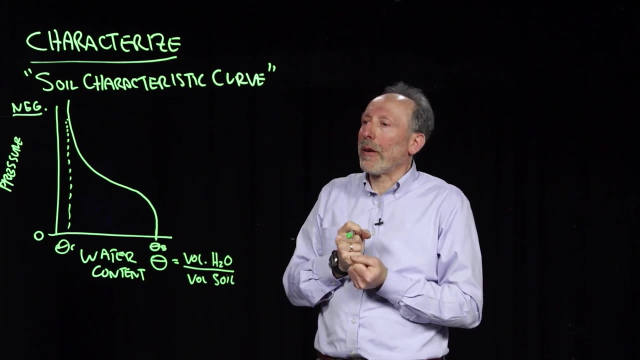 out. So the characteristic curve looks something like this: So this is then saying that somewhere here we get to a residual saturation where no more water can be drawn out simply by trying to pull on the water films. What's that mean? That means that the water films are breaking. 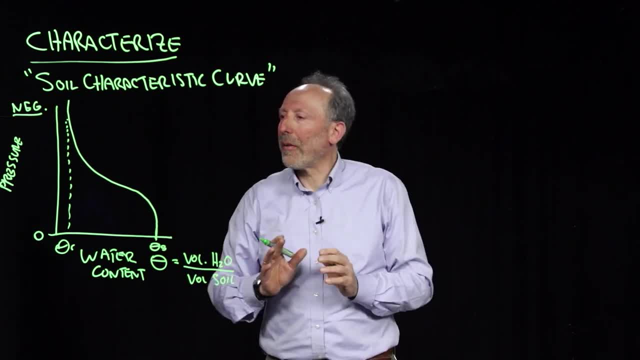 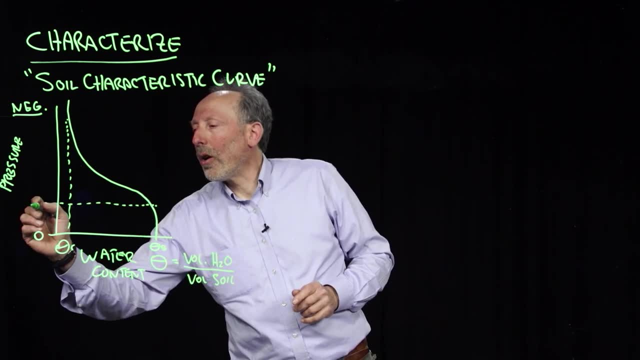 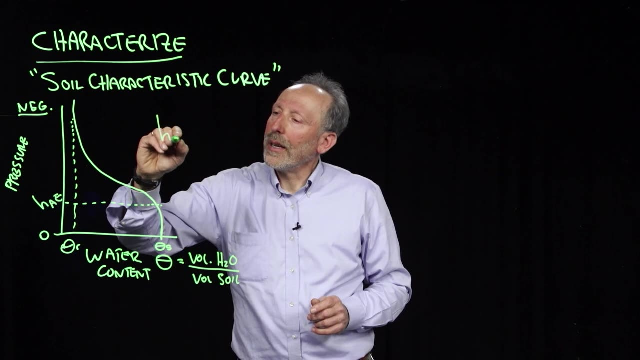 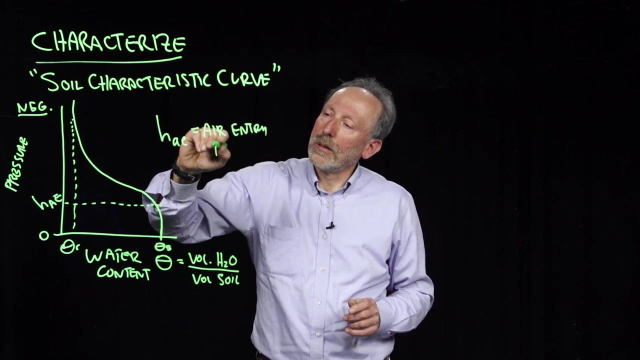 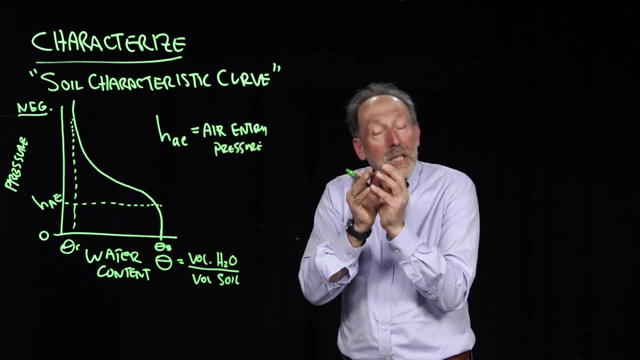 down and we have isolated elements of water throughout the soil. So we have theta sat, theta residual, We might call our air entry pressure, Excuse me, So we call HAE is going to be the air entry pressure. That's when the water had been fully filling the pores and when, essentially, 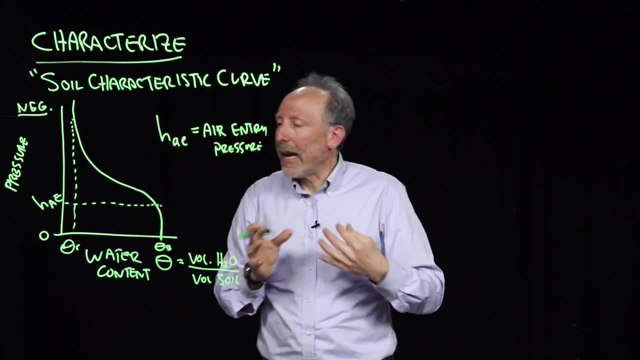 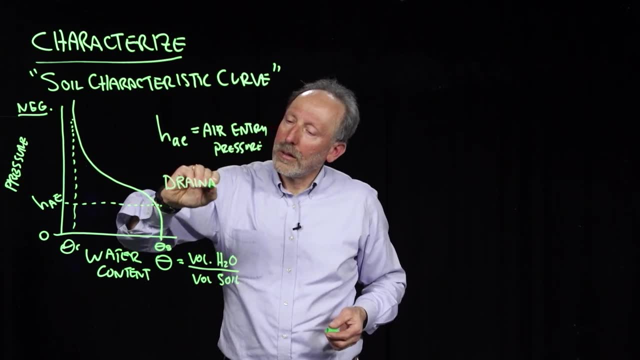 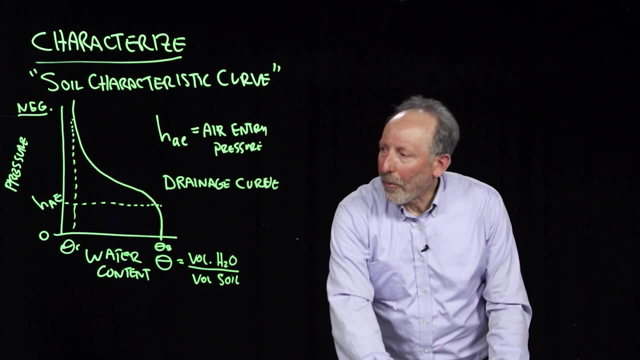 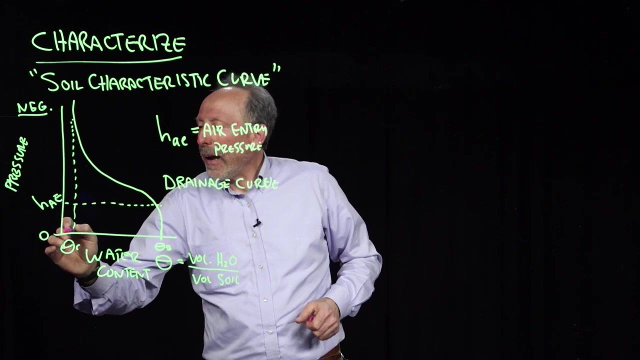 the largest pores start releasing their water because the air is entering, And this is called the drainage curve. Now, when we're draining, it goes this way, but we can also fill the soil, And so when we fill the soil, we might start from absolutely dry soil In this case. I'm going to start. 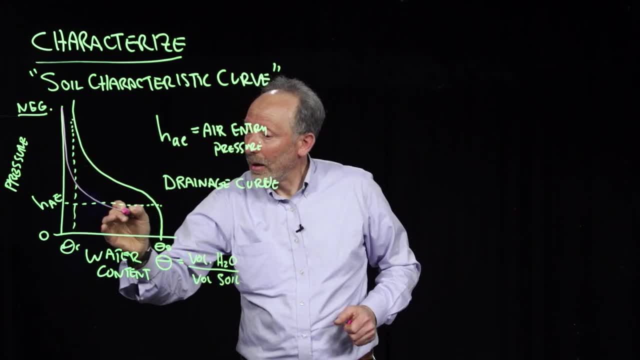 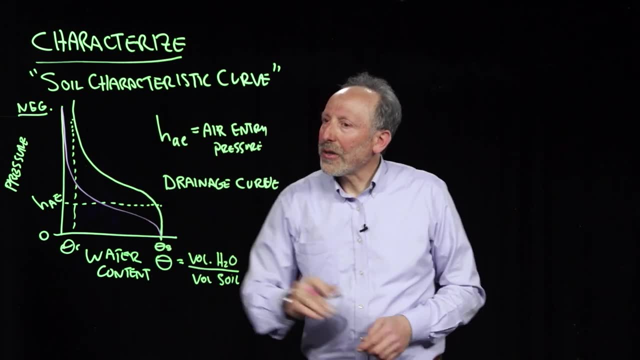 from dry soil And I'm also going to end up with fully saturated soil, But what you can see is that these two curves are separate. So I'm going to start from dry soil and I'm also going to end up with fully saturated soil, But what you can see is that these two 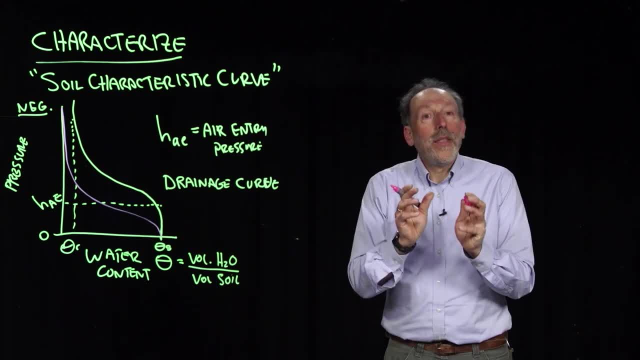 curves are separate. So I'm going to start from dry soil and I'm also going to end up from dry soil and I'm also going to end up with fully saturated soil And so when the wet that's saturated, that means that soil that has started saturated and dries versus. 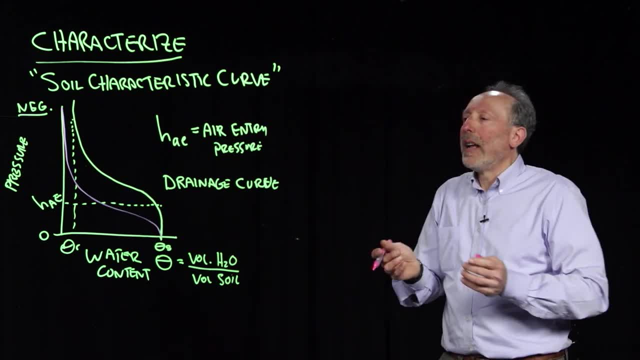 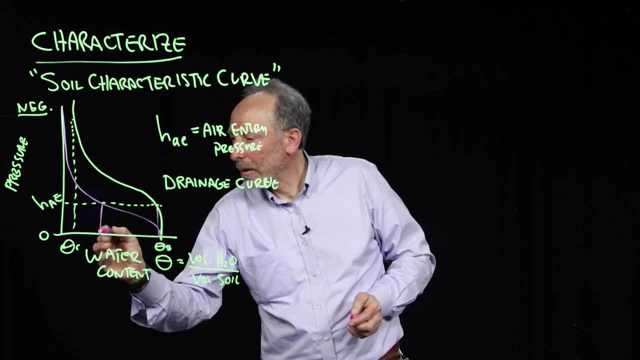 soil that has started dry and saturated ends up for the same pressure, might have very different moisture contents. This is called hysteresis 來說, And hysteresis is very important, as you can see, because what the plant does is the 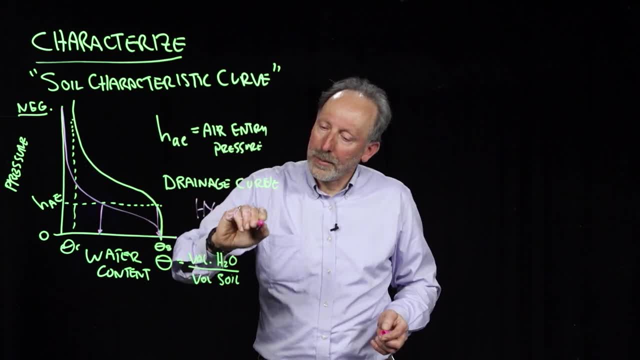 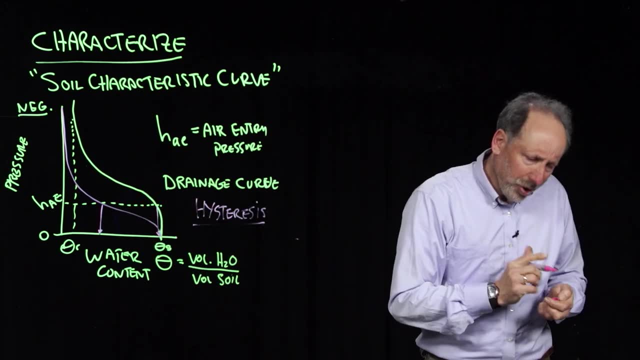 plants need all the fuel for this, Absorbing various siblings of the soil with a thermal situación and 티er-seizer апę Symphony. is that thisrament? when you do that but you're clearing water up with a conventional do is the plants apply pressure, They try to pull water out of soil, But if the soil 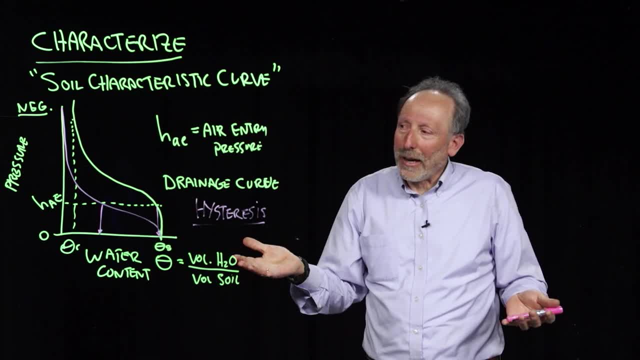 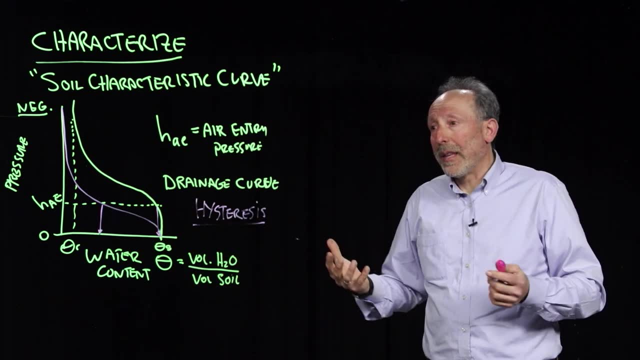 was starting saturated, the plants might have a very easy time getting the water out, Whereas if the soil had started from dry conditions, that same water content would be at a much lower water content. So this hysteresis is a fundamental piece of the soil characteristic. 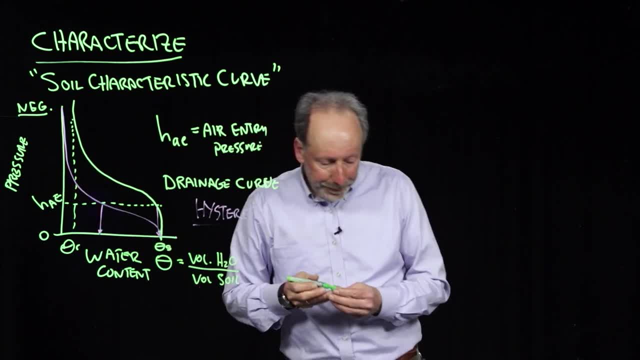 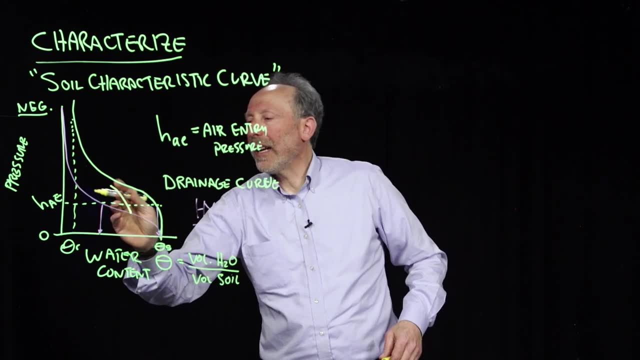 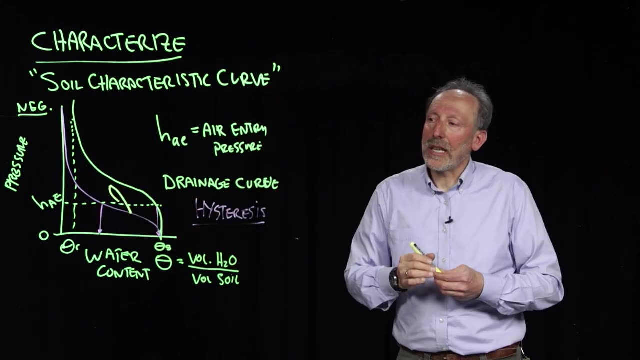 curve, And if we were wetting here- so we're wetting here and then we decide to drain again- we can actually get another curve coming from that curve. And then we say: oh no, let's start drying again So you can get these systems of hysteretic curves, so that you can have. 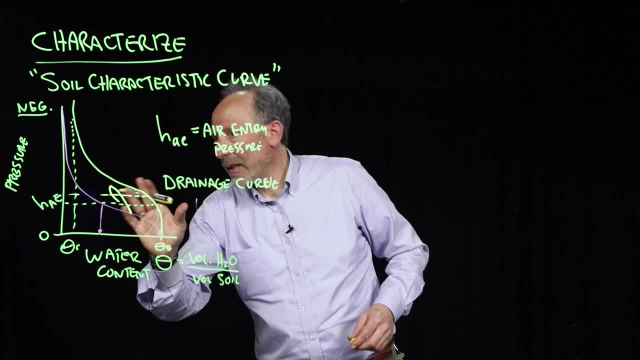 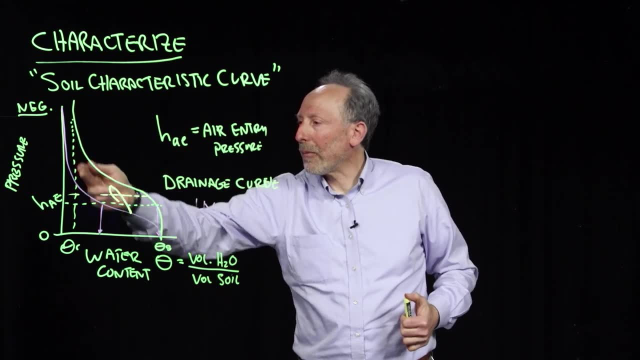 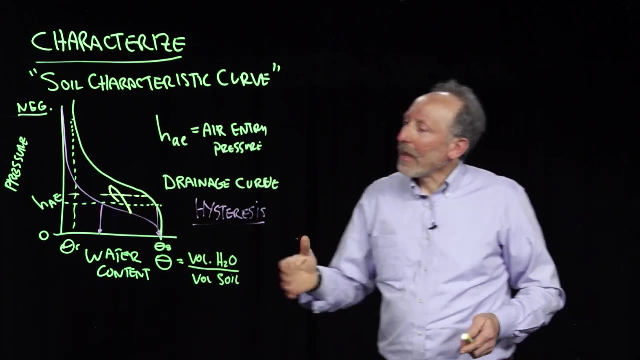 almost any number of moisture contents for that, given same pressure. So when we characterize soils, first off we say what are the characteristic curves of this soil that define when it's fully saturated draining and when it's fully dry wetting, And then with those two curves we can predict everything else. And this is: